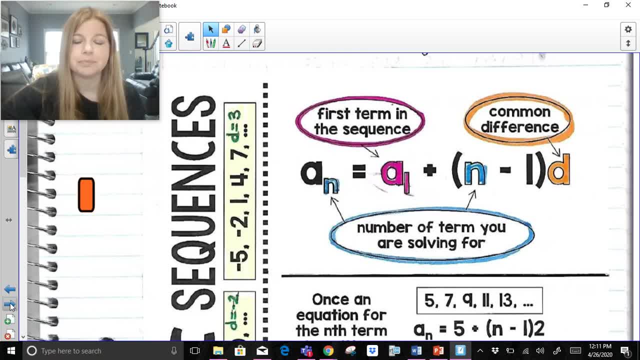 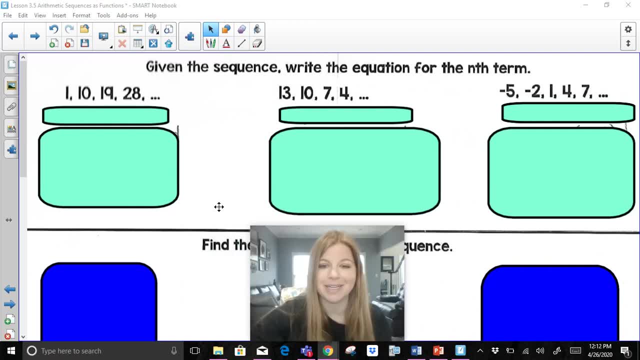 thinking where does this even come from but let's take a look here's what we're gonna do it says given the sequence write the equation for the nth term now what's really nice about writing an equation for an nth term it means that you get to leave n in the formula and so I really just need to know my a sub 1 and I need to know my common difference D so if I give you the sequence 1 10 19 28 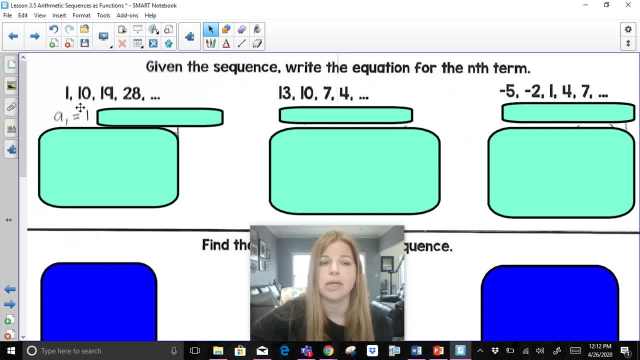 the a sub 1 for this sequence is 1 it's the first term the common difference D would be whatever I see it's increasing by so here I see it's increasing by 9 so my D is a positive 9 now here's that 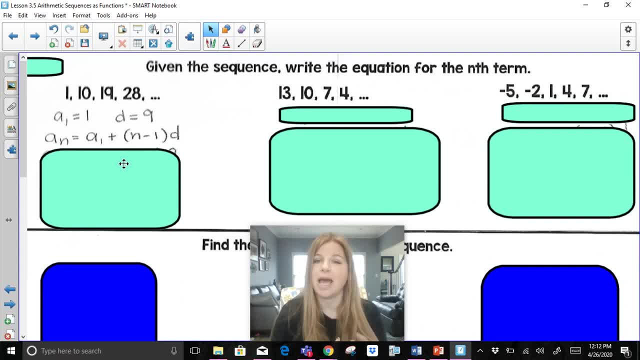 formula a sub n equals a sub 1 plus n minus 1 times D I get to now substitute in 1 for a sub 1 and 9 for D now when I do that I'm writing this equation for the nth term when you get to write an equation for the nth term it means wherever you see n you just leave it there you don't need to plug anything in 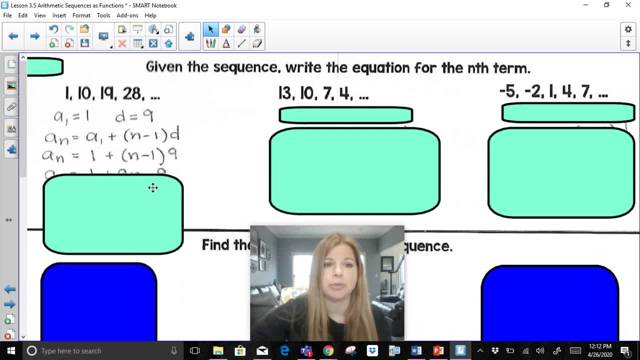 I'm gonna clean this equation up a little bit so I'm gonna go ahead and distribute that 9 so if I distribute 9 to n minus 1 I get n minus I had 9 n minus 9 with that one in front and then this is what my final equation would look like after I combined like terms this would be the equation for the nth 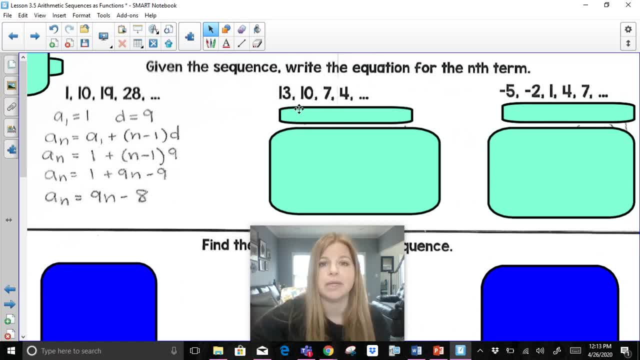 term given the sequence let's try the next one 13 10 7 4 the first term of the sequence is 13 the common difference D here is that it's subtracting by 12 three, so d is negative three. Here is my formula. I go ahead, I substitute in my 13 for my a sub one and my negative three for d. I'm going to now distribute that negative three, so negative three 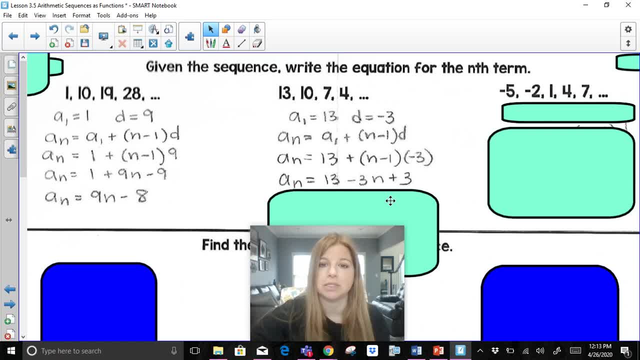 times n, negative three times negative one, which gives me 13 minus 3n plus three. I'm going to go ahead, combine my like terms, and it becomes negative 3n plus 16. Last one, my a sub one is 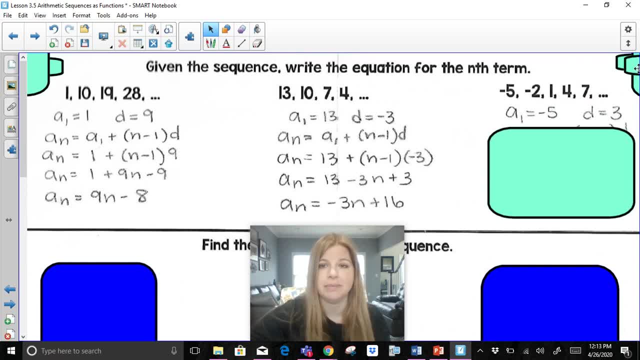 negative five. My common difference d is three. I get to go ahead, substitute my a sub one in for 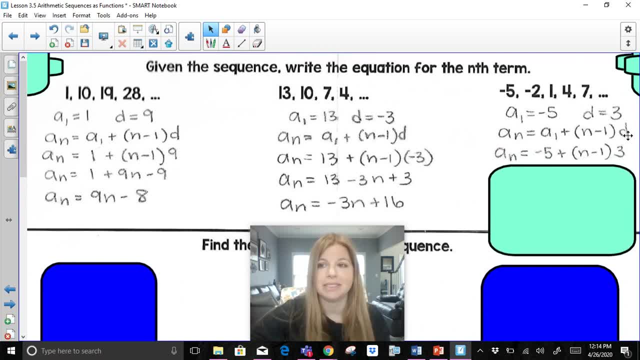 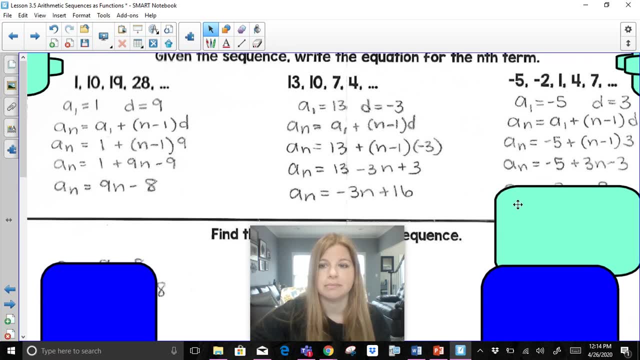 my negative five in for that a sub one. My d is three. I'm going to go ahead, distribute that three, and then combine my like terms. That's it. Those are my equations. And again, when it says to 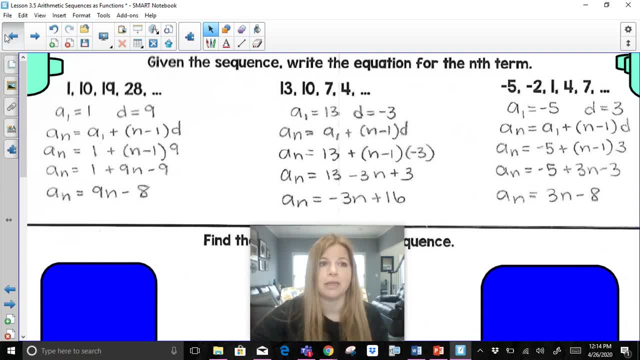 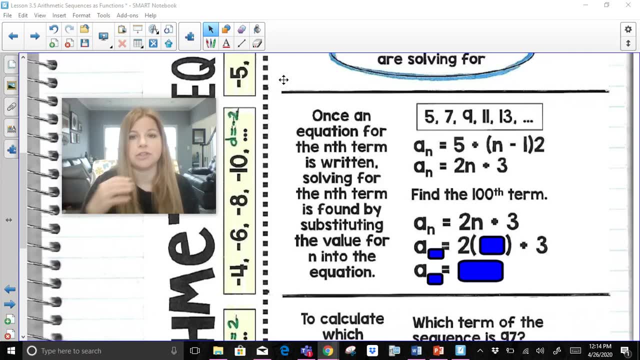 write the equation for the nth term, that means you should have n in your final answer. So now we're going to take a look at what it means to write the equation for the nth term. It means to then do the next step. So it says, once an equation for the nth term is written, solving for the nth term is found by substituting the value for n into the equation. So if I gave 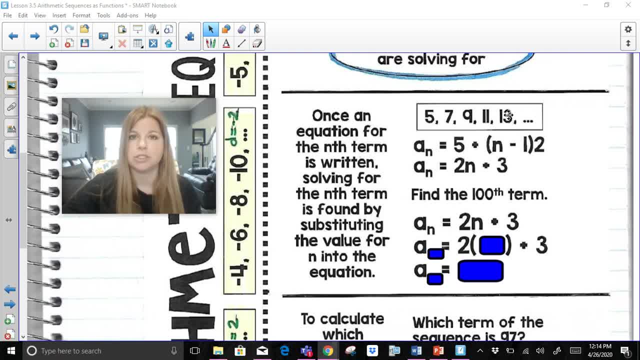 you the sequence 5, 7, 9, 11, 13, and I said to write the equation for the nth term, we would plug in a five for my a sub one. We see it's increasing by two, so my common difference here is two. And let's say I already did all the distributing and combining like terms, and I get this. a sub n equals 2n plus three. If I then said to you, find the hundredth term of the sequence, what that means is every place I see n, which is two places here, I substitute that hundred in. So a sub 100, which means the hundredth term. It doesn't 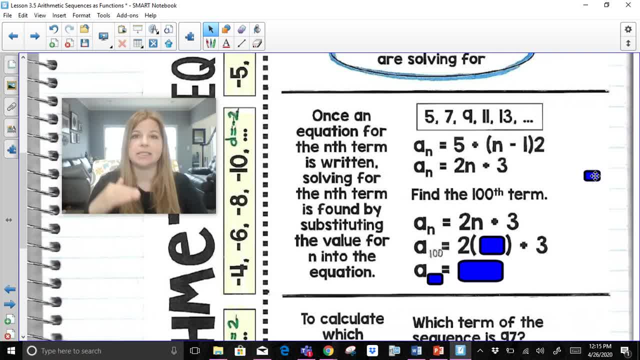 mean a times a hundred. It's not a hundred a. It's just simply a sub 100. So this is saying the hundredth term of the sequence is equal to two times. I plug in that same value for n, two times a hundred plus three. So the hundredth term of the sequence, a sub 100, is equal to, 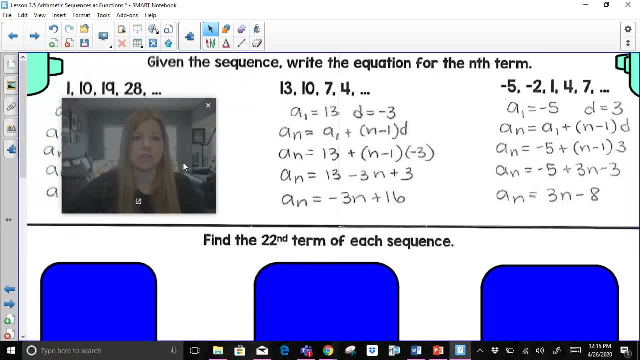 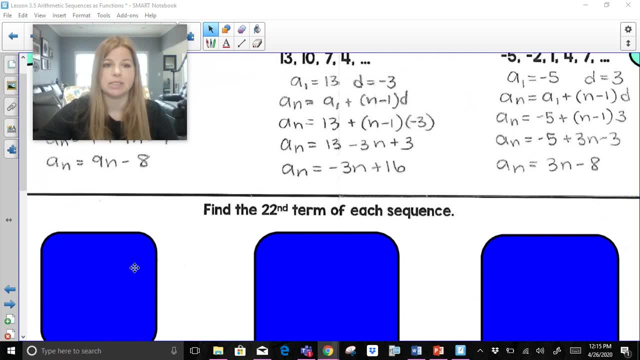 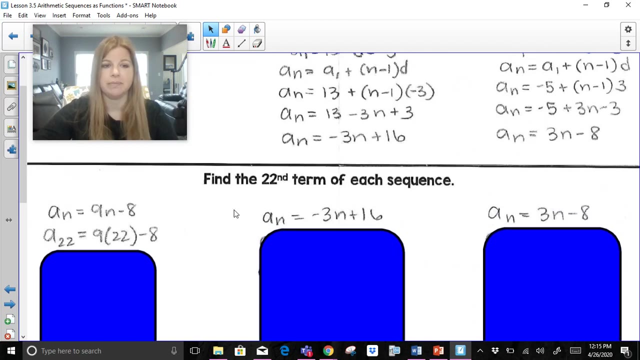 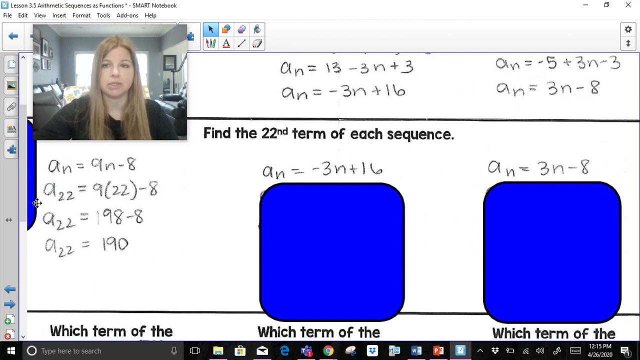 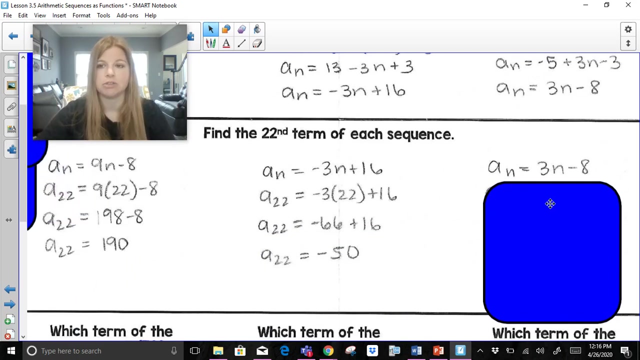 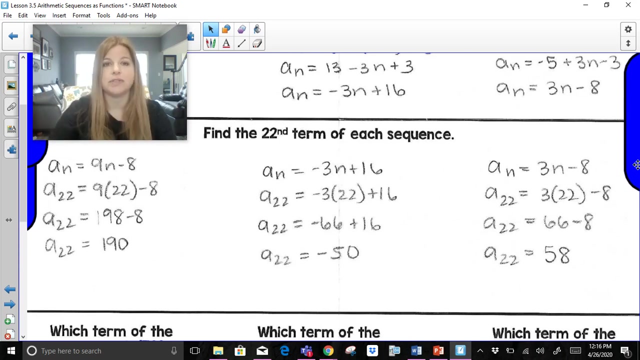 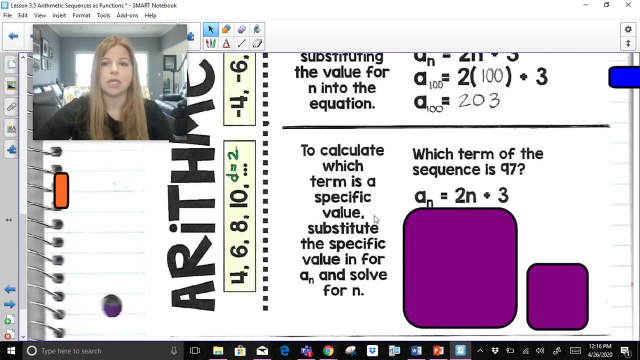 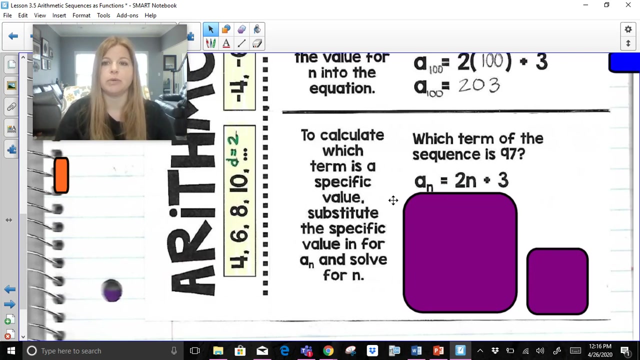 two hundred and three. So now, if I go back to these equations that I created here from these sequences, and I now say to you, find the 22nd term of each sequence, I would take this equation that I created, and I would substitute 22 in for where I see n. So here, if I go ahead and I take those equations from up top here, the ones that we already started to create, and I go ahead and I plug 22 in, I'm really just doing my basic sequence. So I'm going to go ahead and I'm going to go ahead and I'm simplifying, and notice what the result is. A sub 22 equals 190. So that's saying the 22nd term of the sequence is 190. If I wanted to find the 22nd term here of that middle sequence, okay, I'm just substituting that in. Notice the a sub 22 stays the whole time. I'm not changing it. I'm not doing anything else with it. And then here, if I plug in a 22, I'm just doing my calculations and evaluations on the right-hand side, left-hand side, just stays a sub 22. Very easy. So now the last thing I need to show you is, what if I told you, hey, here's the sequence 5, 7, 9, 11, 13, which number term of the sequence is 97? And you may be saying to yourself, okay, well, I can count that out, right? So 5, then 7, then 9. But do you really want to go all the way to 97 and figure out which term of the sequence has a value of 97? No. 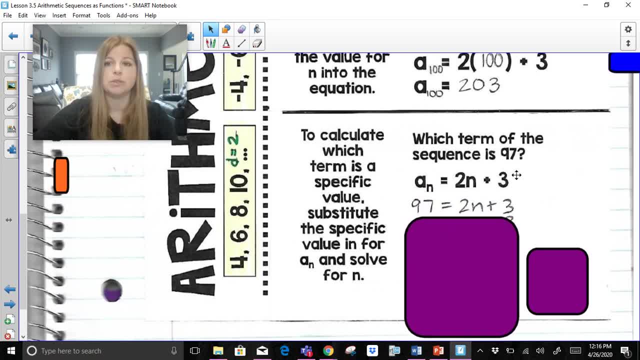 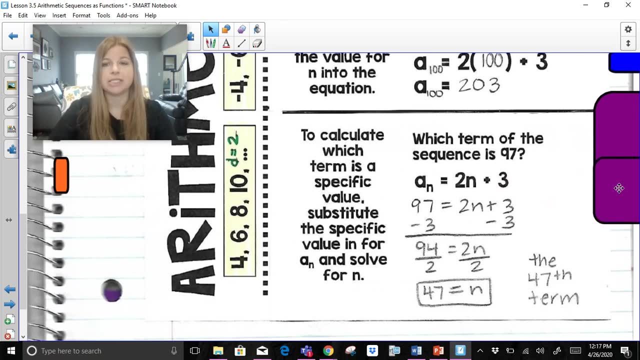 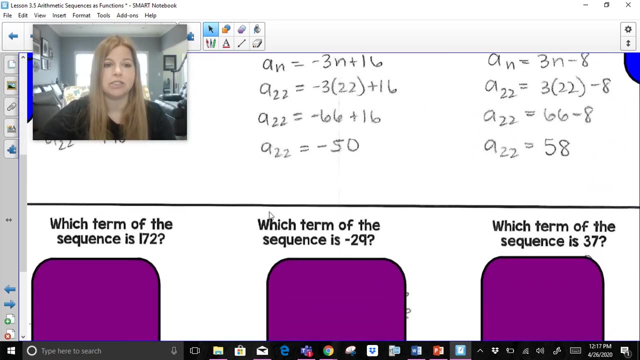 The way we solve it, we solve for that number term is we substitute 97 in for the entire a sub n value. So if 97 gets substituted in for a sub n, and I solve for n, and I end up getting 47, that would mean the 47th term of that sequence would actually be 97. So if I take a look here, and I show you, and I said to you, which term of the sequence is 172? And let's say I had this formula that I created, and I said, okay, I'm going to take a look at this formula, and I'm going to 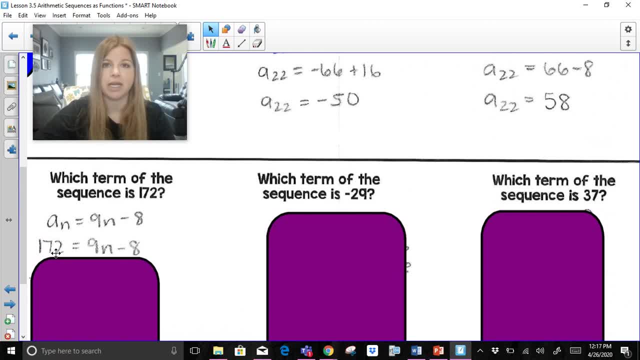 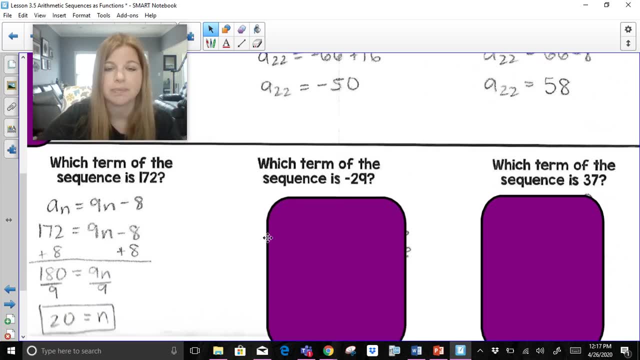 from above, I would then plug in 172 in for a sub n, and then solve for n, and I would learn that 172 is actually the 20th term of that sequence. Okay, again, which term of the sequence is negative 29, I would take that formula that we created, plug in negative 29 in for a sub n, and then solve. 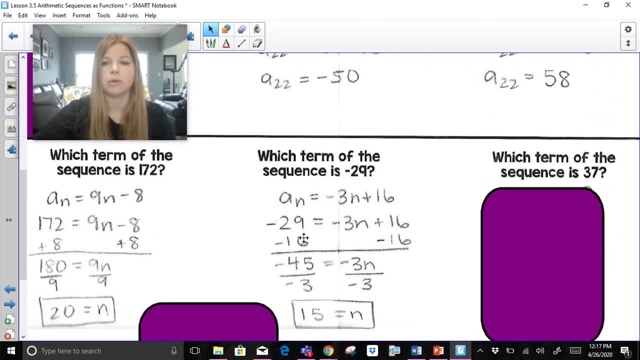 The solving point at this point is very easy for us, because we've already dealt with our equations.